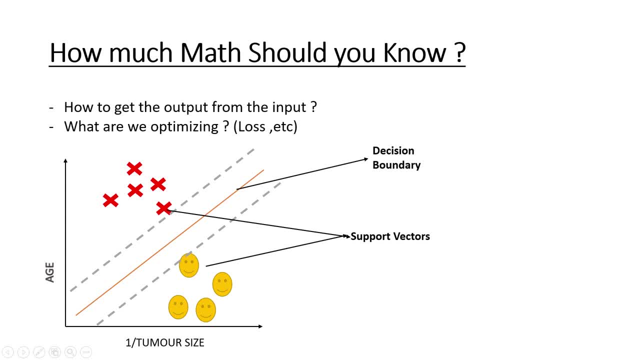 between the two classes. So we're going to proceed with the maths for that. So how much math should you know? In any machine learning model, you should understand a how are you getting the output from the input, Which means once you have come up with a decision boundary and then you have a random. 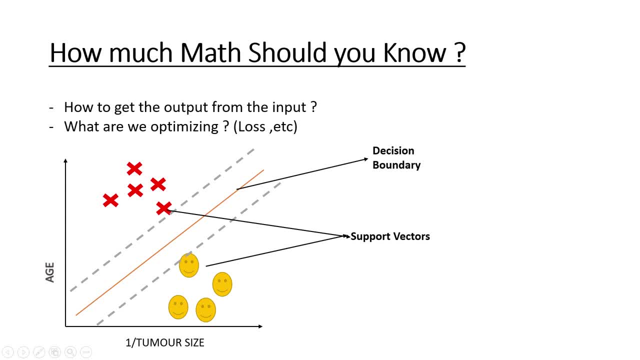 point. how do you determine which side of the decision boundary does this point lie on? You should understand the maths behind that right, Because every time you use the model dot predict function in your programming right, That is what happens internally. It's. 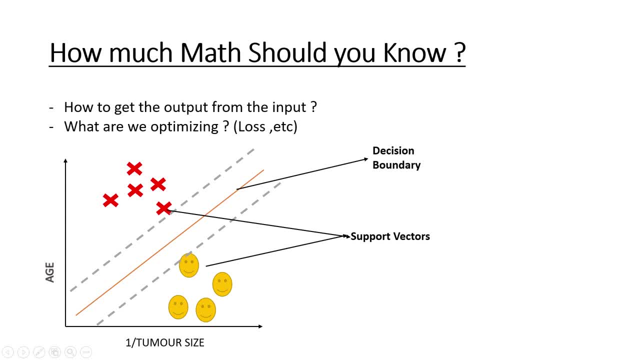 calculating the output for a given input. Second is: what are we optimizing? You need to know this because this is the factor which will decide which machine learning model is better than the other. For example, if you have two decision boundaries, there needs to be some parameter so that you. 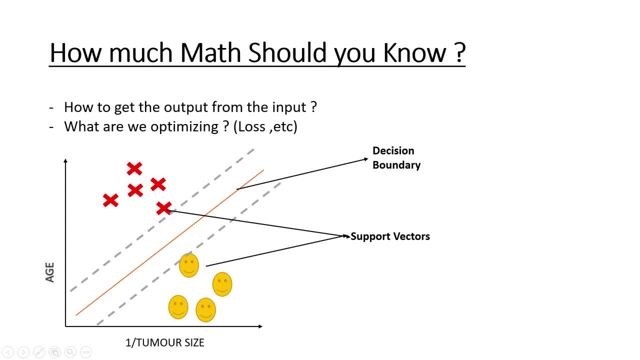 can compare the efficiency of these two models, right. What are you going to optimize? There's going to be some equation that you're trying to maximize or minimize, always right. So let's look at that. Starting with, how do you get the output from the input for that you? 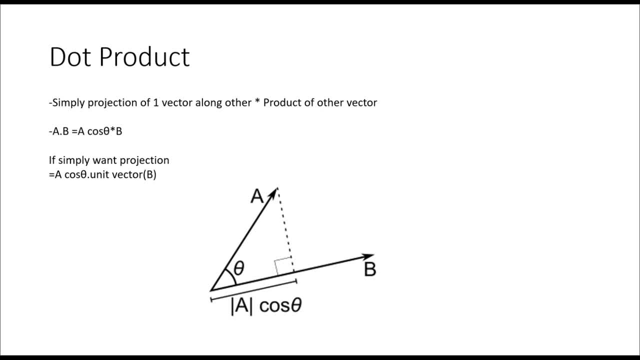 need to understand a concept which is called as the dot product right. What is dot product? Simply put, it's the projection of one vector along the other into product of the other vector. The projection of one vector is equal to a cos theta, where a cos theta is the projection. 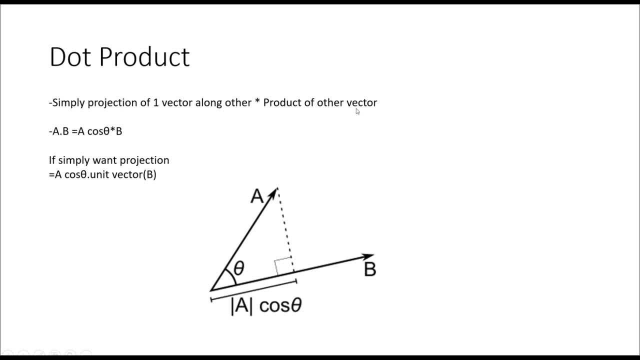 of a on b right. You can imagine that someone who's putting a torch right He's throwing some light on top of a and the shadow which is cast on b is nothing but a cos theta. It's the projection multiplied by b. Now, if you're simply interested in the projection of a and 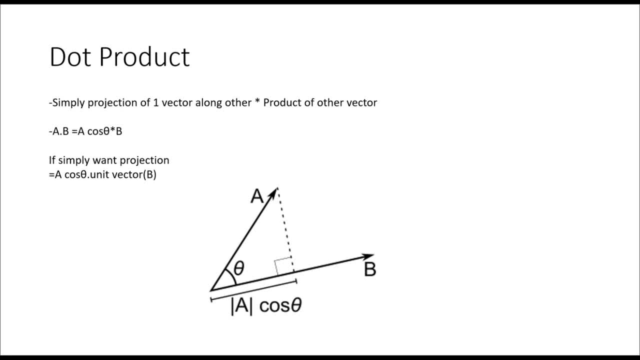 you don't want to multiply with the magnitude of b, you can replace the equation as a cos, theta dot, unit vector of b. So what are you going to do now? You're going to return the project in the direction of b, however with the magnitude one right. So if you simply want the projection, you can. 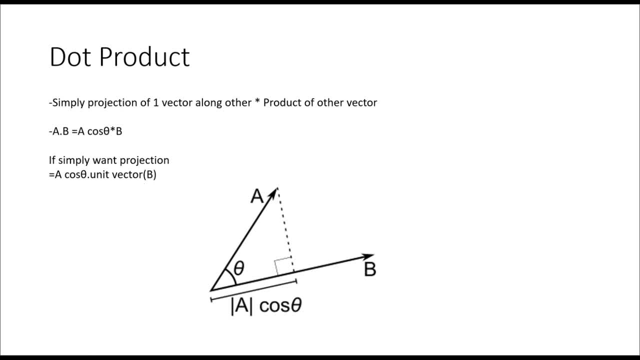 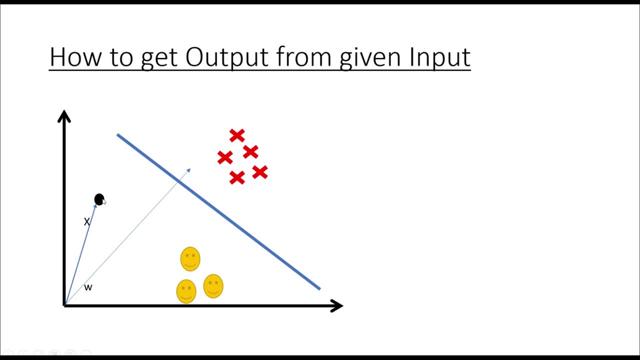 use this equation. So how are we going to use this in SVMs? So let's consider that you have a random point right x, which I have shown, and you want to find which side of the decision boundary does it lie on. Is it above the decision boundary? 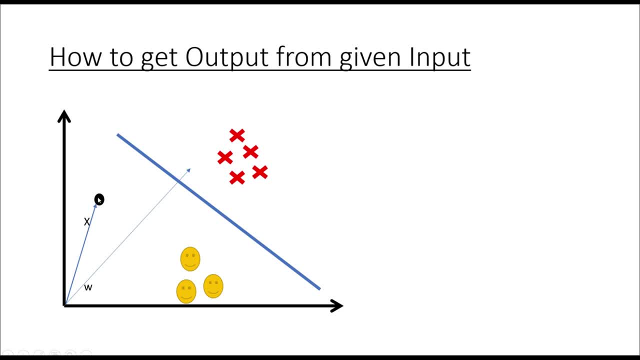 or below it, Right. So what we do in SVM is very simple. So we assume this point as a vector x. So what we do is we take this and we assume it is equal to a cos, theta And x, right. and then we will take another vector, w, which is nothing but the perpendicular along. 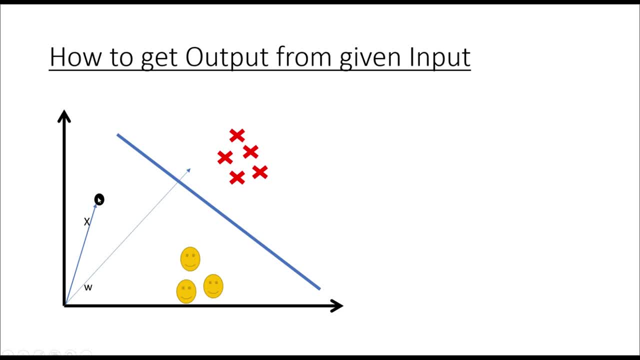 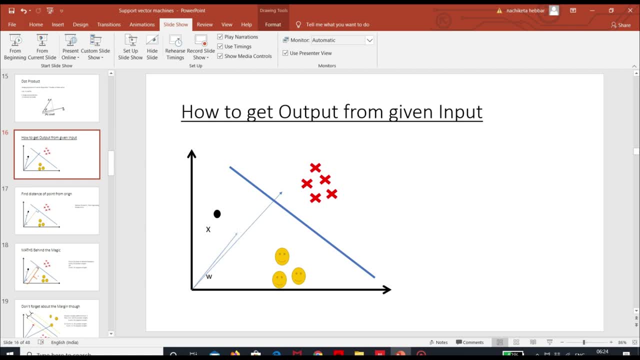 the decision boundary right, and now we take the projection of this random vector on w right. So it looks something like this: basically, the distance from the origin to the point where the perpendicular is intersecting the decision boundary would be known. right could be some random value, say b, right, and we can simply take the projection of this random. 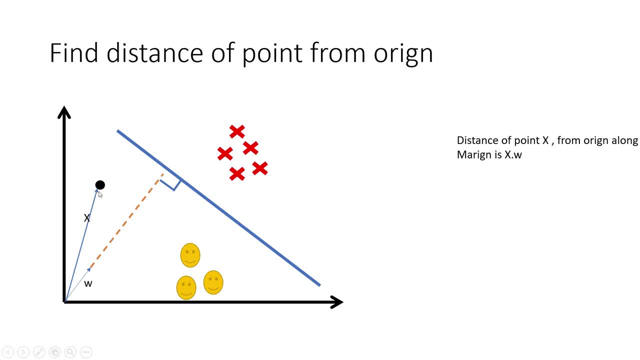 vector on the perpendicular and then compare the distance right. So equation becomes something like this: projection of the vector on the perpendicular is nothing but x, dot, w, right, and if that projection is equal to b, that means the point is on the decision boundary. if it is greater than b, then it means it is some positive sample. let 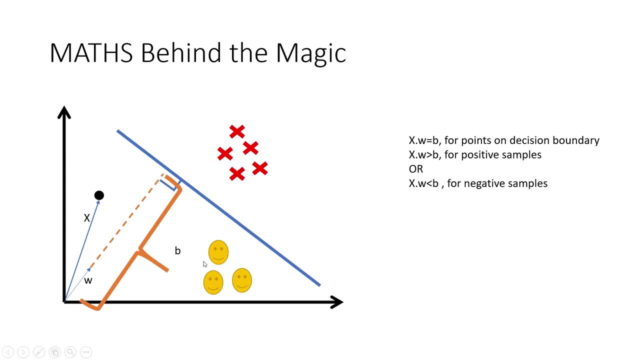 us assume this cross as positive sample right And if it is less than b, then basically lies on the lies below the boundary right for negative samples, right. why are we taking the dot along the perpendicular right? basically, you want to find the distance of this vector from the decision boundary right and there are infinite. 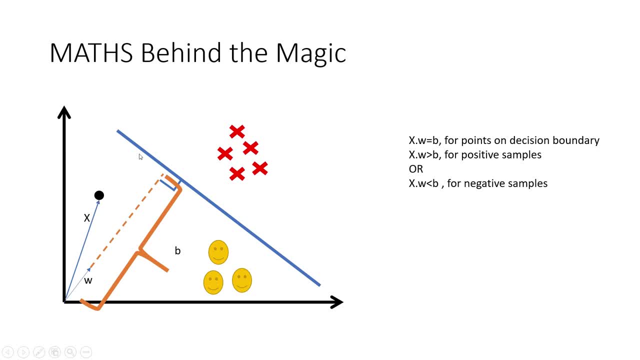 points on the boundary to measure the distance from. So that is why we come to a standard. we simply take the perpendicular as the reference, right perpendicular on the decision boundary, and then take projections of all other points right On the perpendicular and then compare the distance right. so I hope it is very easy and 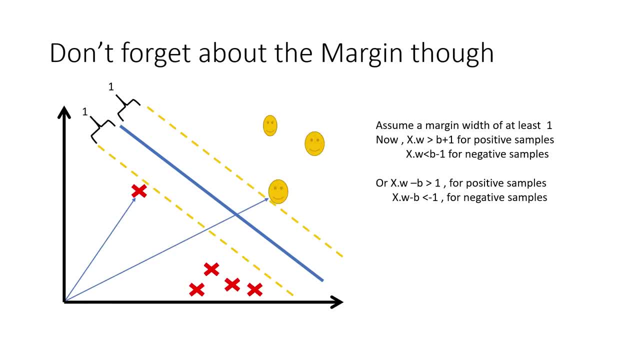 logical so far. now you have to incorporate the margin as well. right in decision boundary you have the margin width as well. so when we have the margin right, the point should not only be lying across the boundary, it should be lying across the margin. so in and in SVMs. 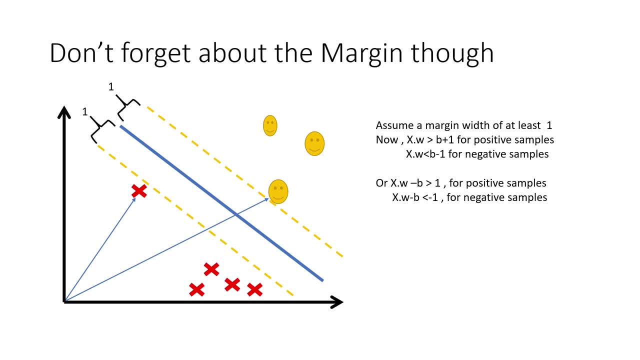 we assume width of 1, right At least that we assume that the margin should be at least one universally, from decision boundary it can be more, but one is taken as a standard. So now in the same equation becomes extra that better than B plus 1 for positive samples. 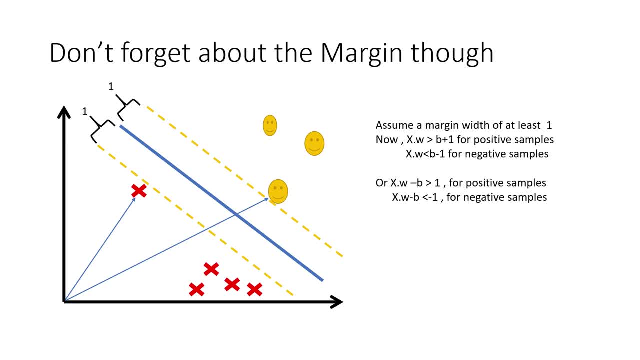 which means you are basically saying should not be above the decision only. it should be about the decision only one and unit of the. So for positive examples will get this equation and for negative sample becomes extra w's less than B minus 1.. And we should the change because in every solution 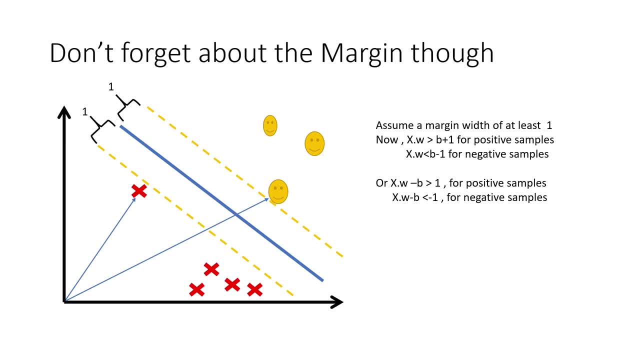 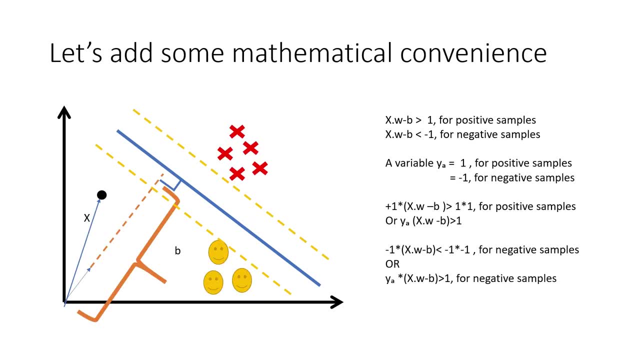 and we should the change. we get this equation by simply transposing the variable b after: okay, so now we're gonna do something to add a little bit of mathematical convenience. right, we're going to introduce a variable called y a, which is equal to plus one for positive samples and minus one for negative. 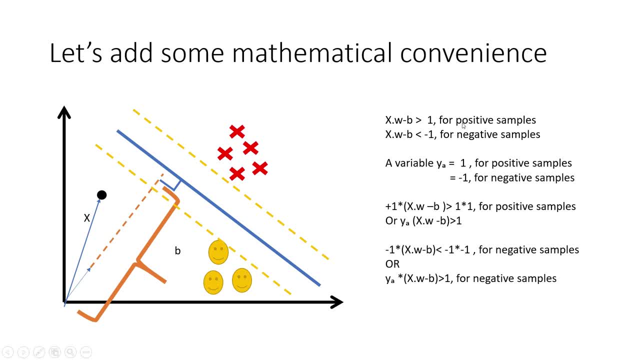 samples. i'm going to show you the reason why we're doing this very soon, but for now let's just multiply both of the equations that we got for positive and negative samples by y of a right. so for positive samples we multiply by plus one on both the sides and you get this equation right: y. 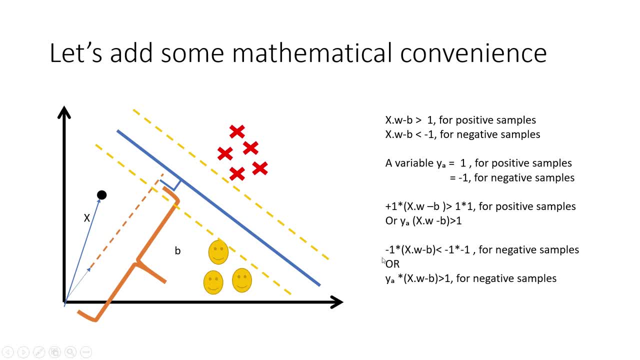 of a into x, w minus b is greater than one. similarly, for negative samples, we multiply with minus one on both the sides and you get this equation. because i'm multiplying by minus one, the sign of inequality changes. and now, if you pay close attention, you can see that both of these equations 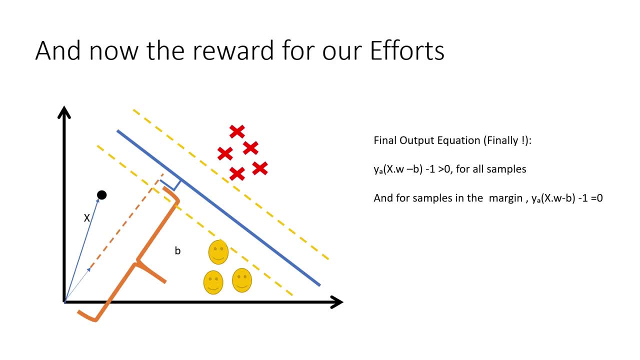 for positive and negative samples is the same. so now we have just one equation that we have to look into you, which is this: right, you can forget everything else- which is y of a into x, w minus b minus one, should be greater than zero for all samples, and if your sample is in the margin right, just on this. 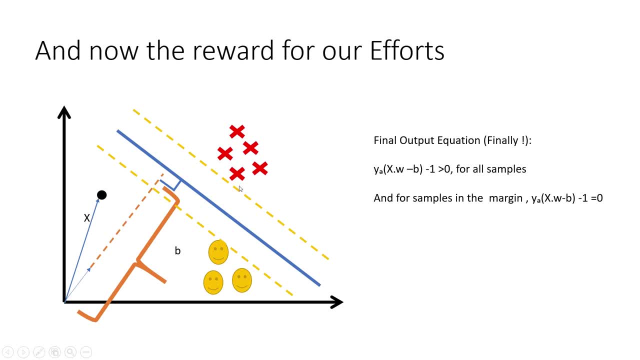 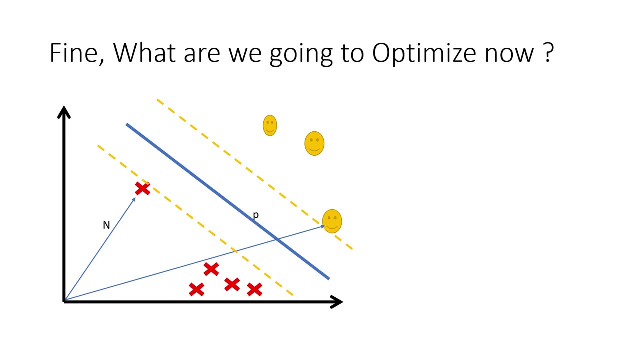 boundary right, this value will be equal to zero, right for points on this margin boundary. now, that was it. that was all you need to know on how to find the output from the input, but we still have to find out. what are we going to optimize? right? and since this is a maximum margin classifier, it's obvious that we have to maximize. 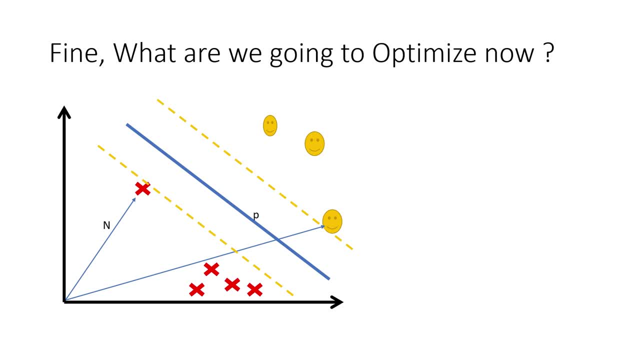 the width. the greater the width of this boundary, the better your svm model. so you need to find out what does your margin width exactly depend upon, right? so let's look into that again. we're going to be using the concept of dot products, right? so for this, i'm going to take two examples. right, say. 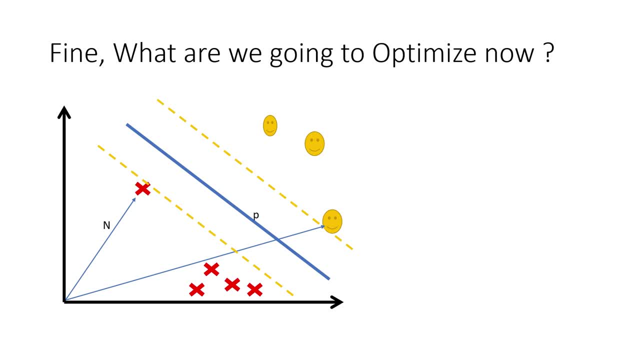 there's a negative point on the boundary right. there's always going to be pound points on the boundaries, which are called the support vectors right. so let's take one in the negative sample, one in the positive sample and represent them by vectors p and n. so this one is vector n and 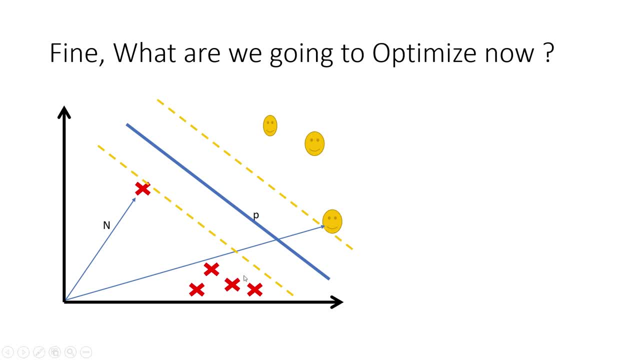 this one is vector p. using these two we have to find the marginlength right. you can figure out from the diagram that we might have to join these two vectors to get something like this right in vector arithmetic this is very simple to calculate if you have to納 method artificial. 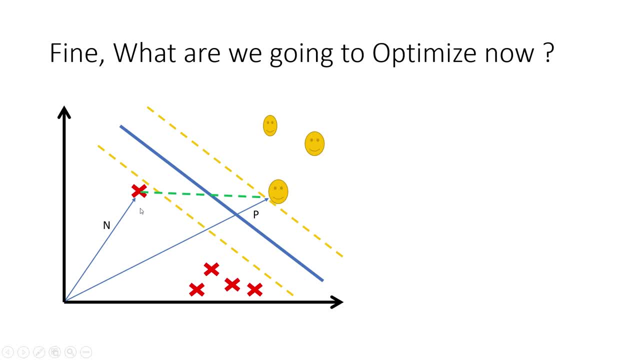 if you have two vectors, then the vector joining them is nothing but the subtraction of the two vectors. so in this case we have this vector as p minus n, the vector joining the negative and positive sample. however, this is not the margin width right, because this is diagonal. we can have 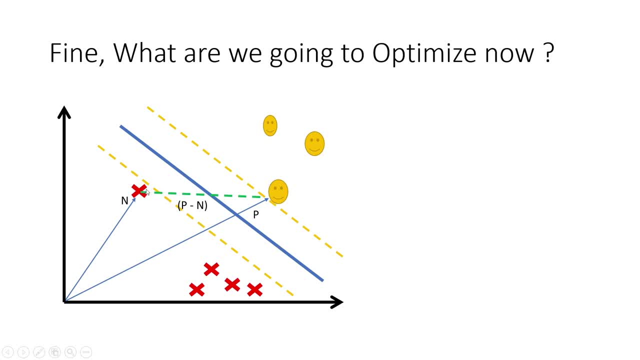 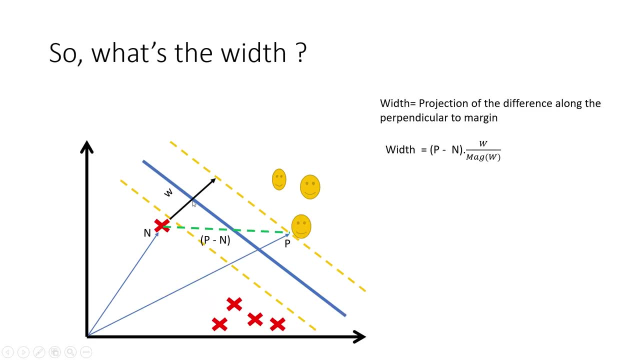 infinite such points right, and which would give us different margin widths. so we are looking for the margin width as the perpendicular to the decision boundary right, which was this. so, again, what we are going to do is we are going to take this dotted line p minus n and take the projection. 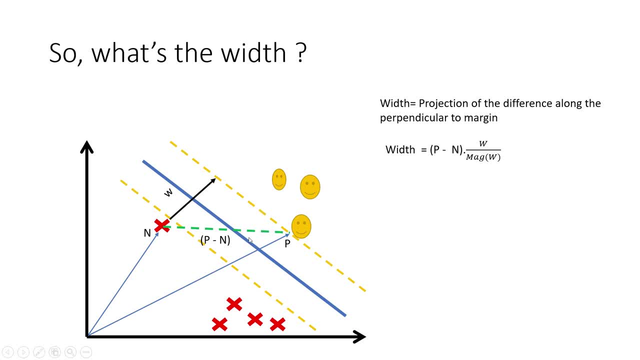 of it along w right. we are basically checking that if this p minus n vector was lying along the perpendicular, then what would have its magnitude been? and it's very easy to calculate that we simply take the projection of the difference along the perpendicular, which gives us p. 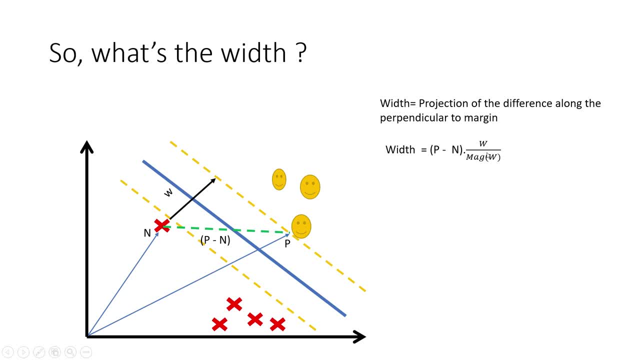 pr minus n n dot. product of w by magnitude of w right. why am i doing this? because we need the projection along the unit vector right. so w by magnitude of w gives us the unit vector along the perpendicular. that's it right. however, there are a lot of variables in this equation and, and coincidentally, 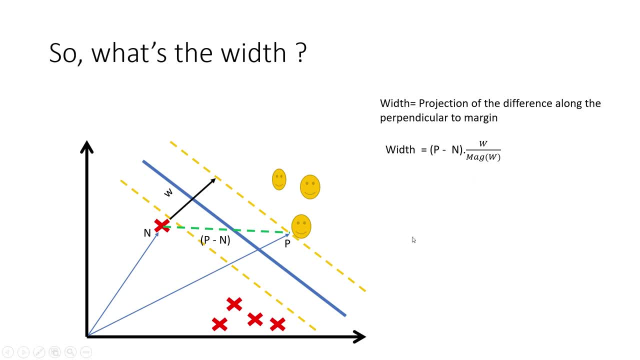 we also know the values of p and n, right, we know the equation for a point lying on the boundary, which is p, and for n as well. so, according to our previous equation, which was this: y into x, w minus b is greater than 1. if you simply substitute y is equal to 1 and x equal to p, you get the. 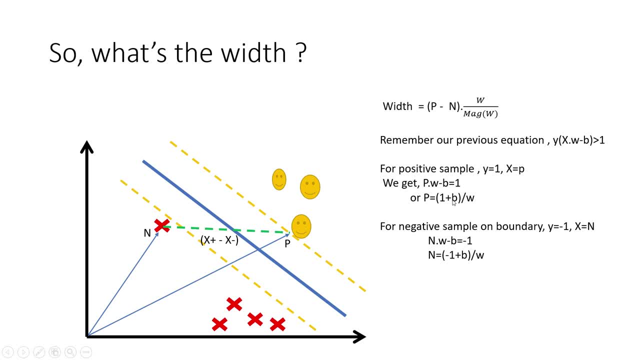 resultant equation for p as this: 1 plus b by w. similarly, for negative samples, take y is equal to minus 1, x equals to n and you get the resulting equation like this. now just the final step, p minus n will give you simply 2 by w if i. if you look at this, b by w and b by w terms will get cancelled. 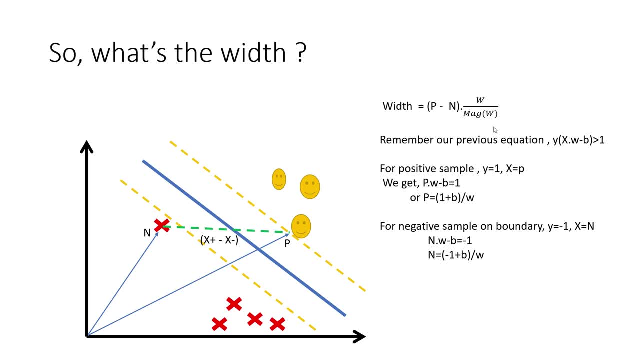 you will have 2 by w remaining and that gets the denominator gets cancelled with the numerator w over here. right, simple math, simple calculation, and you get the final equation looking like this, which is: your width is equal to 2 by w. right, and since we have to maximize the width of the margin, 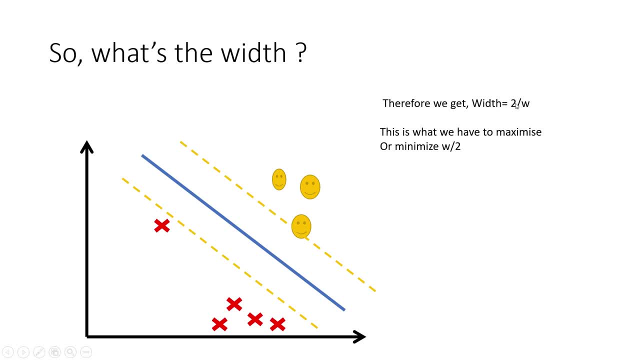 that means we have to maximize 2 by w, or you can instead minimize w by 2. it's the same right. maximizing 2 by w is same as minimizing the inverse of it, which is w by 2 right. so you have done a great deal of the work right around. 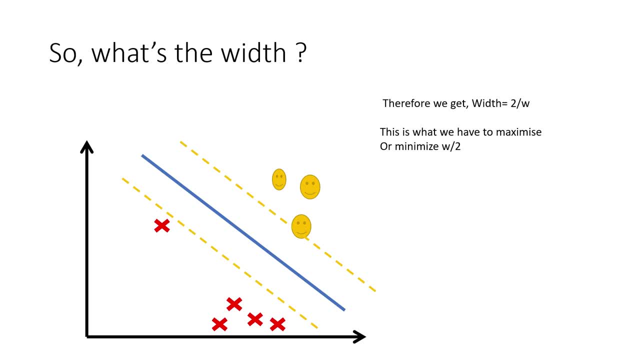 80 percent of the work is done. we know how to get the output. we know what the width exactly is that we want to maximize, which is w by 2. however, you still don't know what the w- w is. you know that w is the perpendicular. 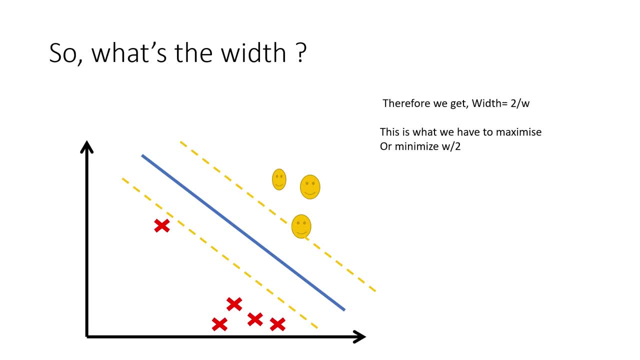 to the decision boundary, but we still do not know what it depends upon right. it could be a very complex functions of all the input samples, or it could be a very weird and random functions. we need to understand what exactly is the width depending upon right. so for that we're going to do. 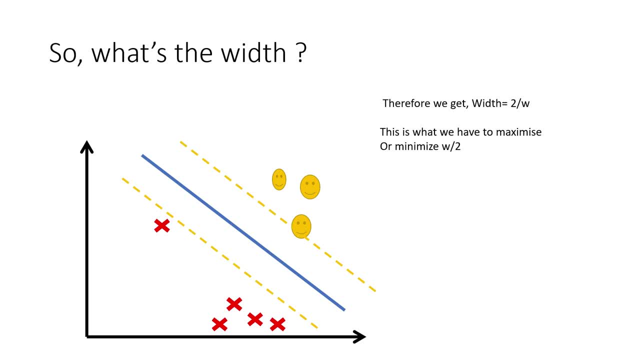 something really interesting. but for now, let me ask you a question. right, so say, we have a certain width of this decision boundary. since i want as large of a width as possible, why not make this width infinity? why not take the margin and place it at infinite distance from each other? right, that's the ideal. 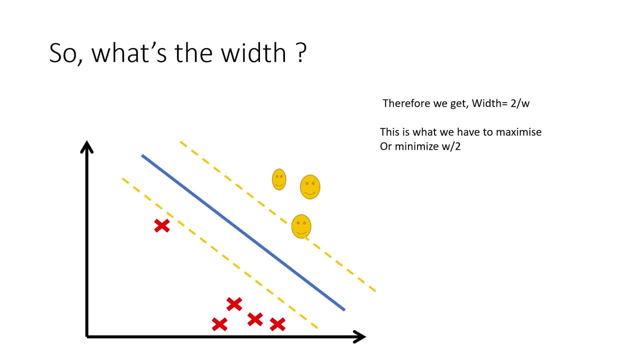 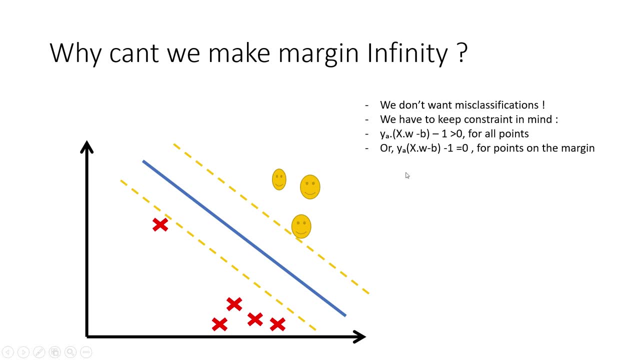 case. right, we could do that. however, we have to keep in mind the constraints as well, because we don't want any misclassification. so we have to maximize the width and we have to satisfy this equation as well. right that the y of a into x, w minus b, minus 1, should be greater than 0 for all. 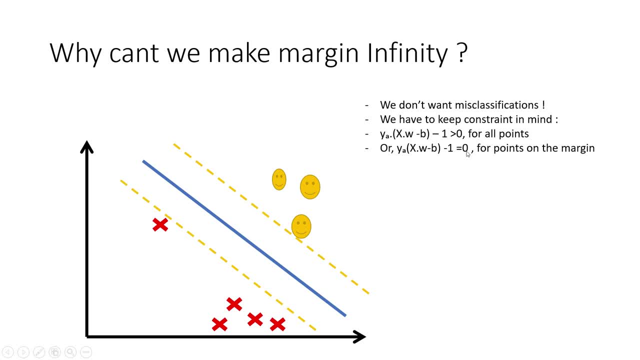 points. or i can say it should be equal to 0 for points which are greater than 0 for all points, just on the margin boundary, right. so we have to do two things parallely: a: maximize the margin and satisfy this equation as well. so i can either, uh say, try a random value of the margin. 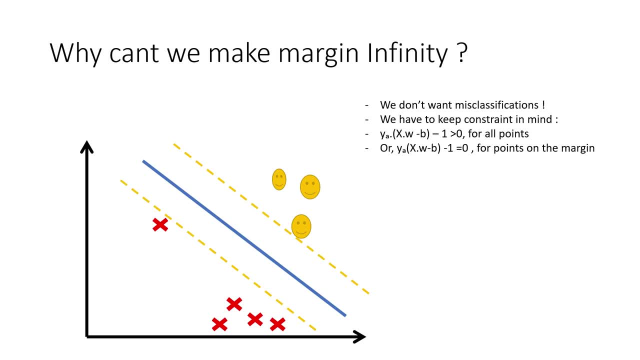 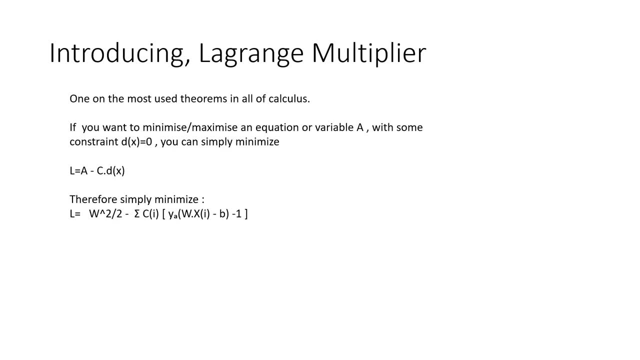 see if it's satisfying the equation, then increase the width and then see it satisfy the equation, which is a lot of stupid work, right? the solution to this is lagrange's multiplier, which is the weapon that we're going to deploy in this case, and it's one of the most popular theorems in calculus. 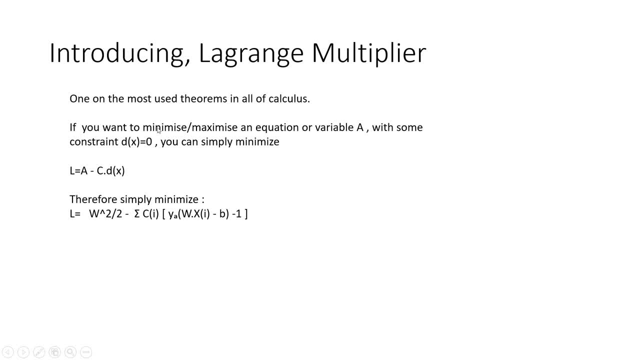 and you see it's simply stated as if you want to minimize or maximize an equation or variable, a right. you want to minimize that term, w, by 2 and you have some constraint. d of x equal to 0. you can simply minimize l, where l is given as a minus c, into d of x. c is some constant. 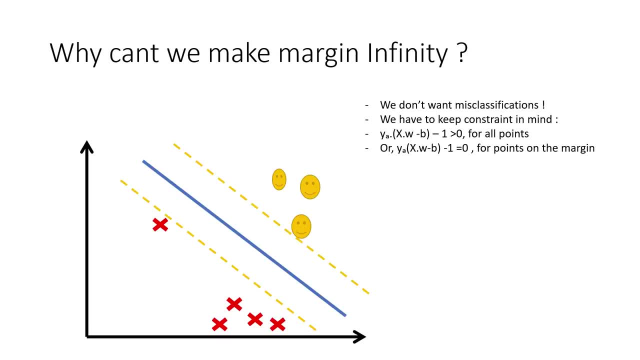 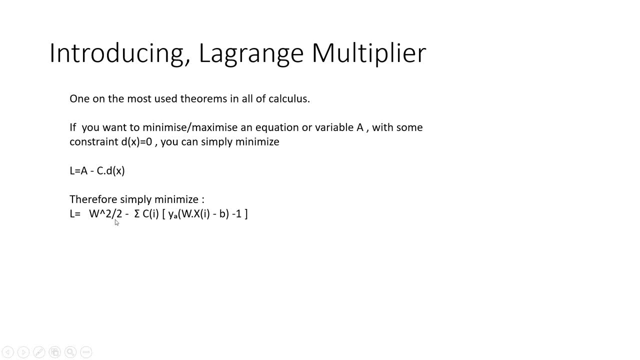 right. so in the previous equation, if you substitute value of a as w by 2, you can see i have written w square by 2 instead of w by 2, right? i'm going to tell you why we're doing that as well. however, just if we write, 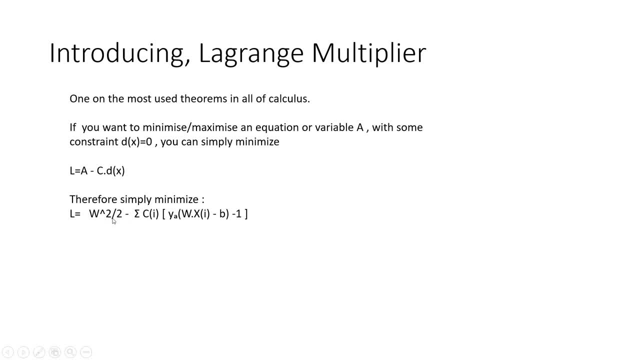 w square by 2, as a right- don't bother about that, i'm going to give you the explanation for that as well- and minus c, and we replace d of x as well. right, which was the constraint. we get this equation right. it might look a little complex and intimidating, but don't worry, it's going to make. 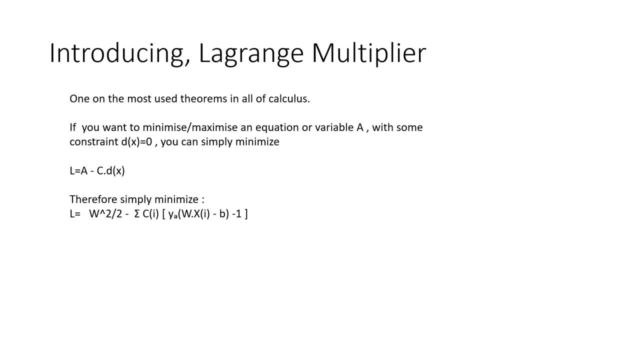 complete sense very soon. so you have this equation and you want to minimize this. how do you go about minimizing such a weird and random equation? right, the solution is very simple: you will go back to a 10 class mathematics and if you have a function like this, right, you're just varying with respect. 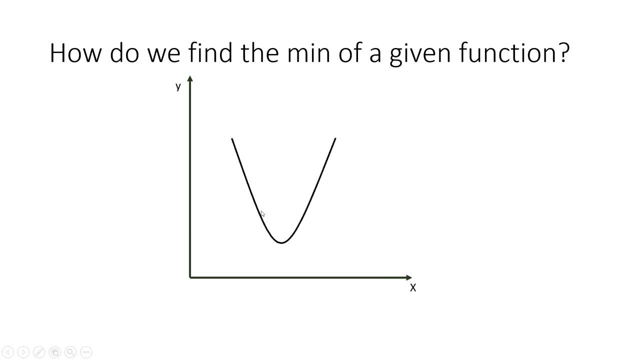 to x and you want to find the minimum. what do you do? you simply take the slope right, which is dy by dx, and equate it to 0. why? because the slope is always going to be 0 at the minimum or maximum point at the peak. basically right, so we're going to use the same thing. 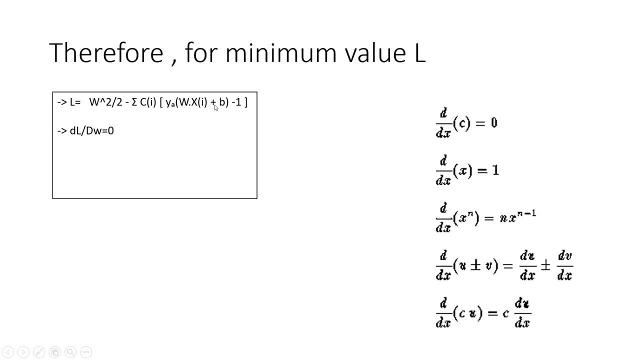 right. we have this equation l right, and we have to differentiate it with respect to w and equate that to 0. right to find the minimum value. right. for those who have forgotten differentiation, i had put up some formulas over here, out of which we are going to be using a few. you can look at that. 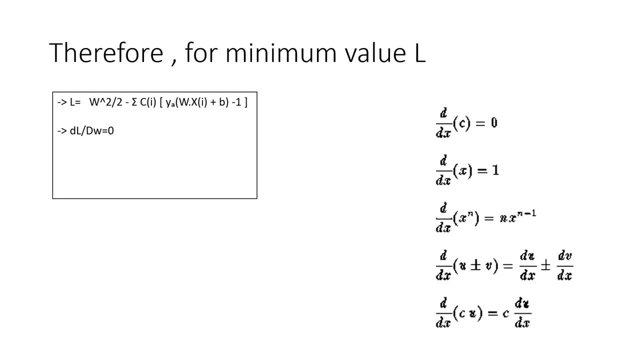 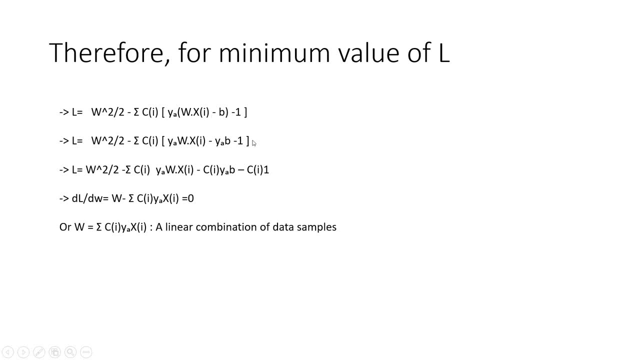 right. so now let's differentiate this. and you have this right. we had l equals to this equation, so i'm simply opening the brackets to get w square by 2 and these terms. now, if you see, if i differentiate it by w, w square by 2 will become 2, w by 2, which is: 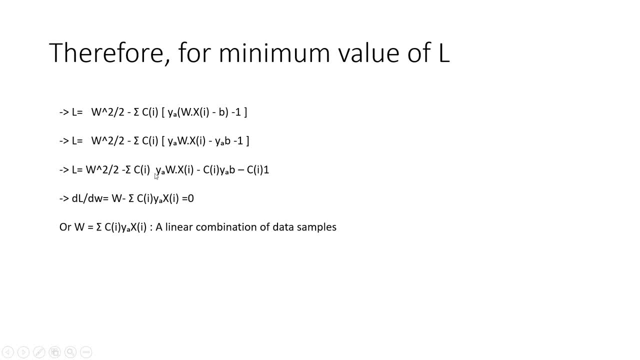 nothing but w. and in this, since all of this is constant except w, we get constant into y of a, into x of i, and since the last two terms are constant, their differentiation is 0 and we get the final result: as w is equal to constant, into x of i, into y of a, which is very interesting. 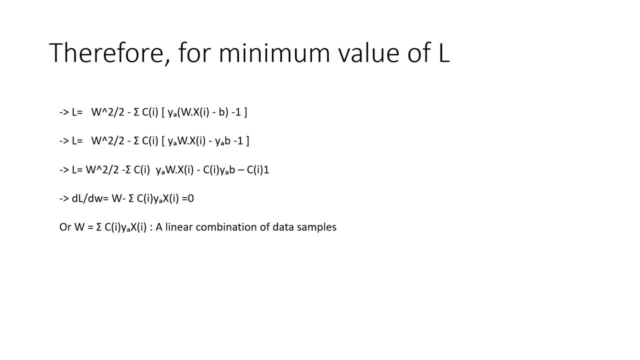 because our width is essentially going to depend upon a linear combination of the data samples. right, it is not any complex functions. you're simply summing up your samples, right? there may be some samples which are playing very high rules. so, for example, when x of i is equal to the support vector. 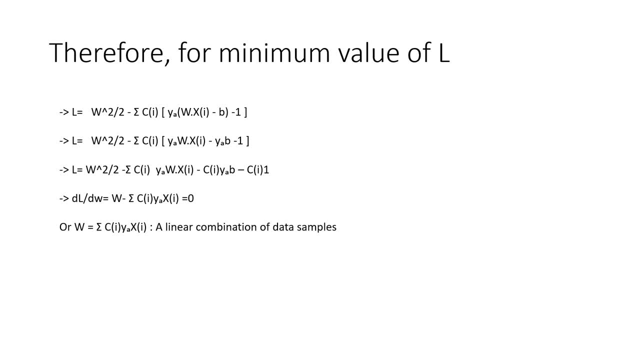 the constant would be very high, a very large number. for other points, which are relatively not important, the value could be less. so this is very interesting to know right. so that was all that we had to know. right, we had done first a how to get the output. now we also know. 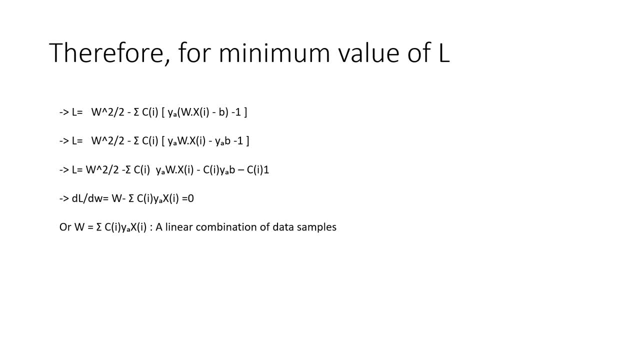 what we have to maximize and what exactly does my margin width depend upon this? all you need to know for the mathematics behind it. now let's look at some things. which makes the svm very powerful. svm even manages to outperform neural networks in a lot of cases, right? so we're going to explore that now. so what we can conclude a you. 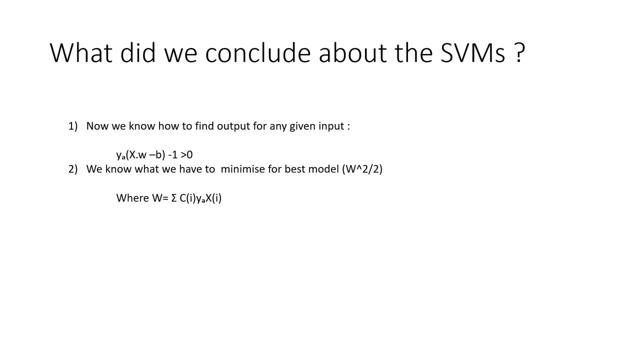 know how to find the output b. you know how to get the best model by minimizing w. to get the best model square by 2. again, i know we had got the value as w by 2, but we are minimizing w square by 2, right, for two reasons which i'm going to tell you later. right, and w is nothing but a constant. 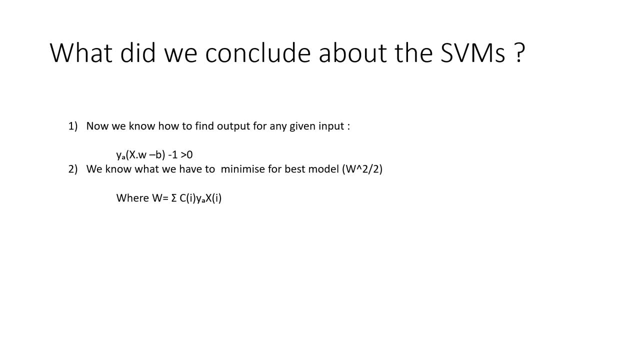 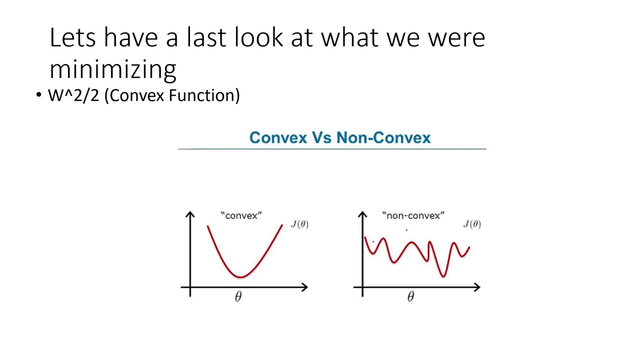 summation of your input samples, right? so let's have a look at what we are minimizing. we had w square by 2. right now in i had replaced w by 2 by w square. now i'm going to tell you the reason why. a it does not matter, right? for example, if i'm minimizing x, the minimum value would be x equal. 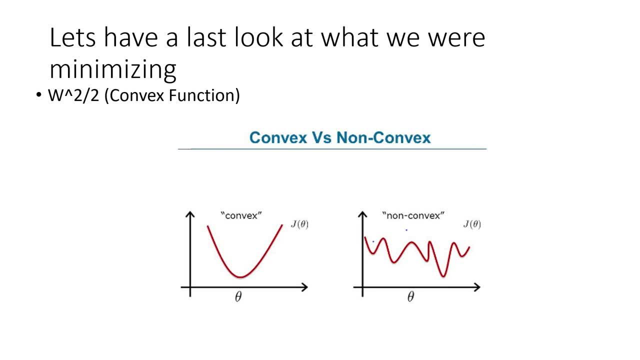 to 0 and if i'm minimizing x square by 2, the minimum value would still be x equal to 0, right? so it's not going to make a difference and it's going to add a lot of convenience, because w square by 2 is a convex function. what is a convex function? 1, which looks like this, which has only: 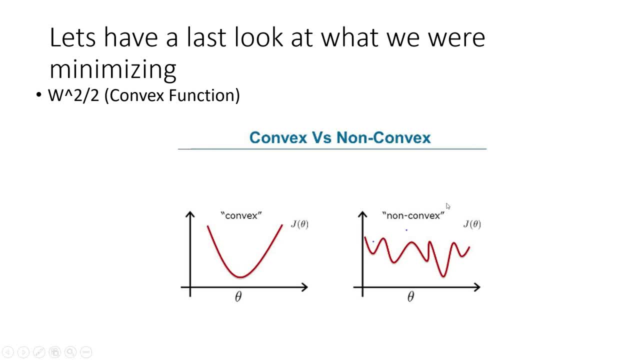 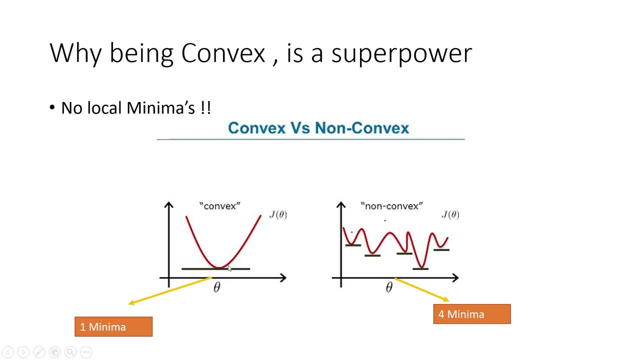 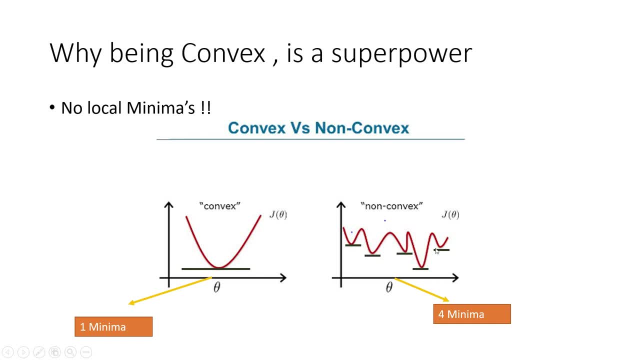 local minimas. what is local minima? local minima is minimum value of the function, however, in the immediate locality, right. so how is how? is it going to be a problem for you? it's going to be a problem because when you get the minimum value of the cos function right, you try to put dy by dx equal to 0. 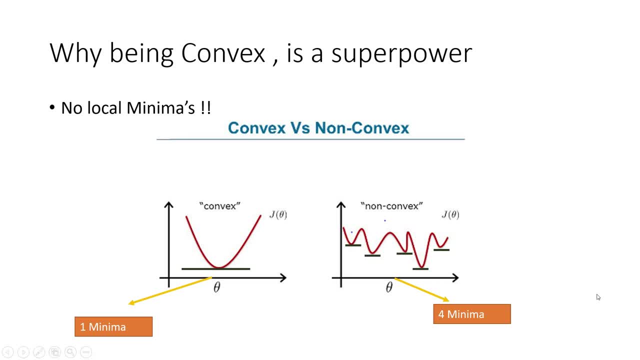 right? so in case of non-convex function, dy by dx is going to be 0 for 5 points and you have no way of deciding which one of them is actually the global minimum, right? so it gets stuck on local minimum. even neural networks gets stuck on local minimum sometimes, right, however? SVM, because it is convex. right, because we are to minimize a convex function. it is never, ever, ever going to be stuck on local minimums. 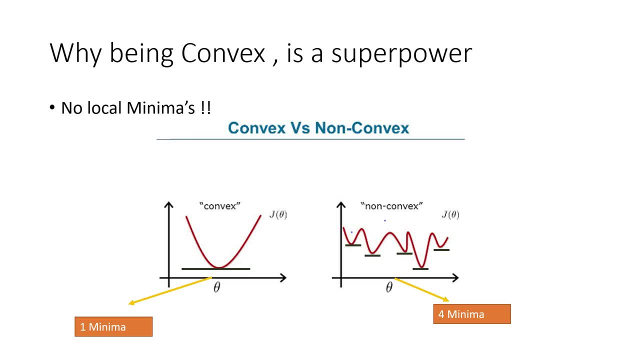 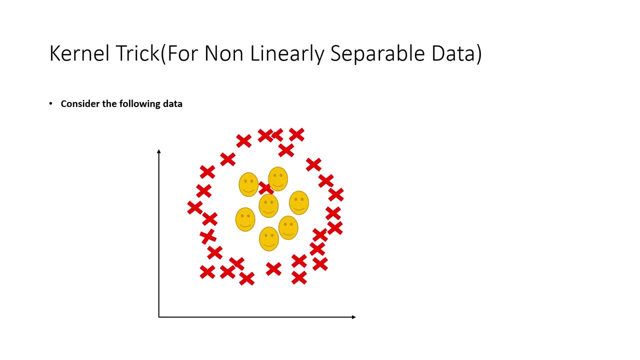 because we are to minimize a convex function. it is never, ever ever going to be stuck on local minimums. That is why it is also very, very powerful and that is why we had written w2 by 2.. The last weapon which SVM uses, which makes it way better than other algorithms, is the. 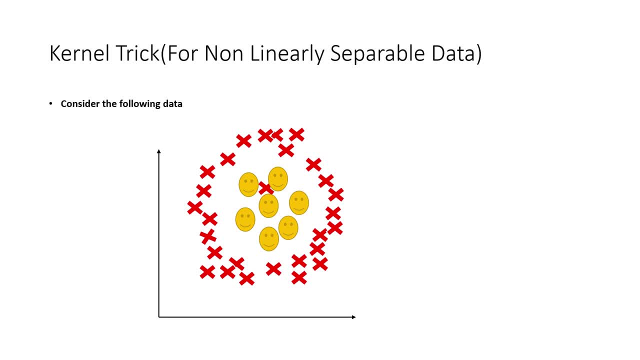 kernel trick which we use for non-linearly separable data. So far we were dealing with linear decision boundaries, which is a straight line. it could have been applied to a plane linear plane as well. however, when you have data like this which cannot be separated by a linear boundary, you can try fitting linear boundaries like: 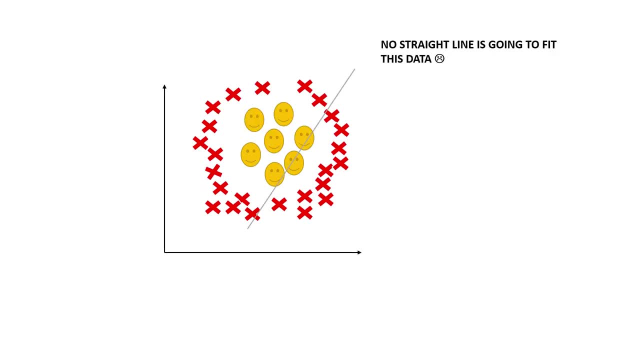 this or this or this, but it is not going to fit the data. You need a circular boundary. you can see from visualizing this, but there is no machine learning algorithm that gives you a circular boundary. So what do you do? Again, SVM comes to the rescue by using a kernel trick which simply transforms the input into: 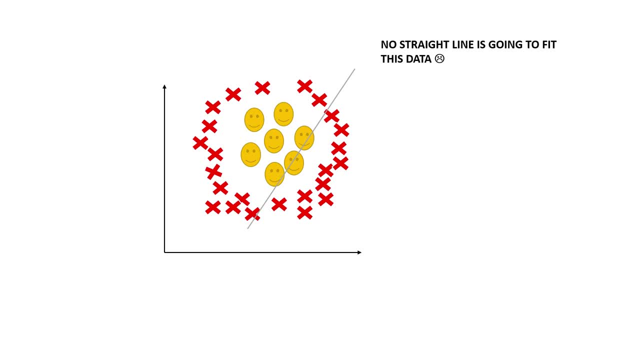 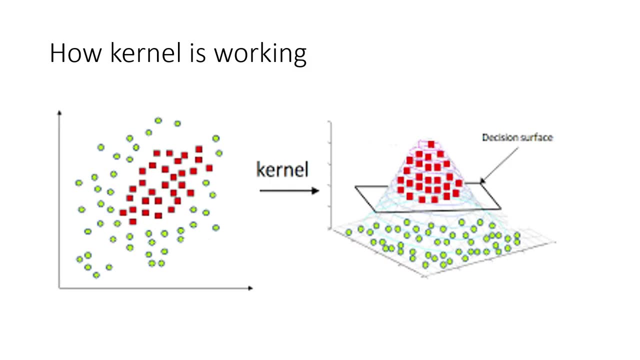 a new dimension where you can separate this data linearly. So what do you do To show you visually, basically what the kernel does is this: You had some points at the center. it is going to take those points and throw them up in. 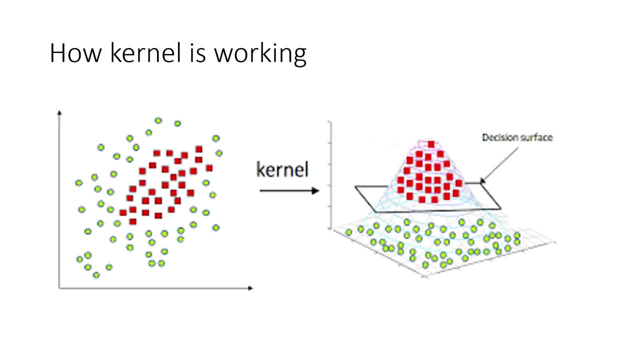 the air and the other points in the boundary are going to remain on the ground, and now you can get a very flat plane, a linear decision boundary to separate these two classes. So even in SVMs we have different types of kernel based on how it is going to transform. 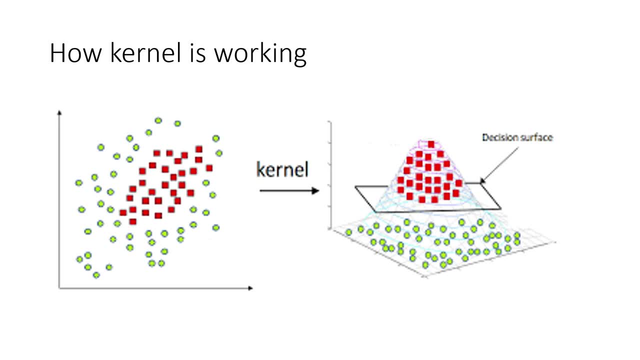 the input. So basic goal of a kernel is to take the input, transform it into a higher dimension where the data becomes linearly separable. right? So there are four broad types of kernel, right? three broad types of kernel in SVM. 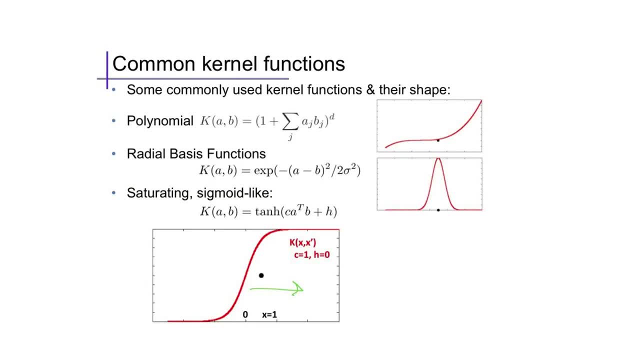 which are. which is this right? you do not need to get confused about the equation. you can even just understand what it is exactly doing, right? So the radial basis function was what we just saw. it is simply an exponential function. 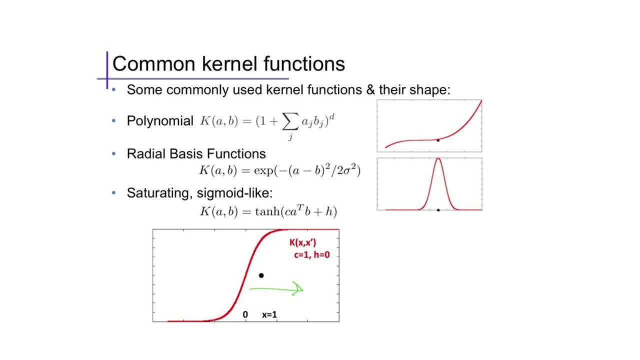 it is taking the input as the data point and what it? what it is essentially doing is taking the points in a certain radius and lifting them upwards right. So whenever you have circular patterns in your data, you would- it would be good to. 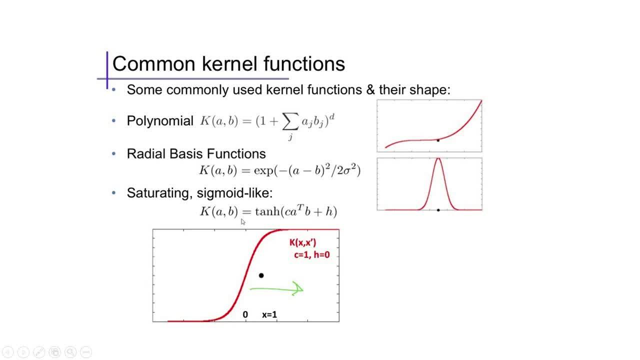 go with this right and the sigmoid function. right is what we saw in logistic regression. it is nothing. it is taking your input again, mapping them to a value of 0 and 1 so that they can be separated by a simple straight line right from the center right.